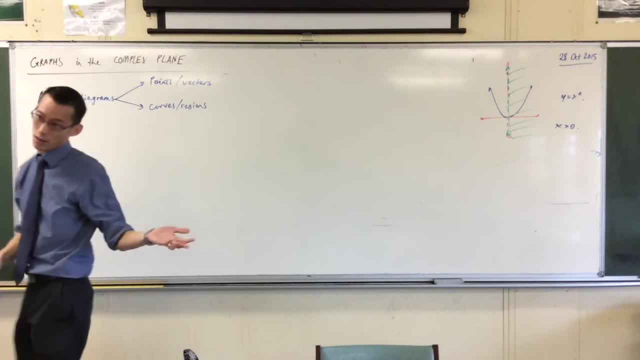 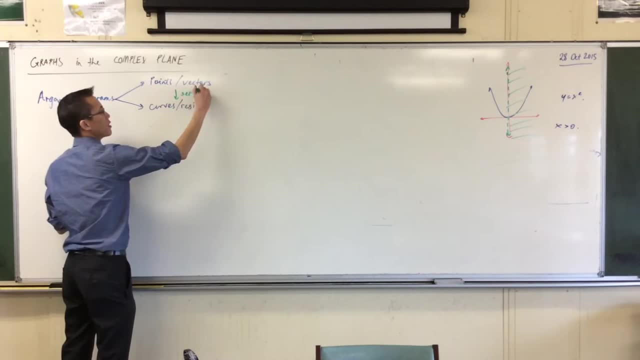 all of those points, every single one of them, satisfies that inequality, Right? So I've got a region or I've got a curve which represents a set of these points or vectors. okay, So we can do it in the Cartesian plane. 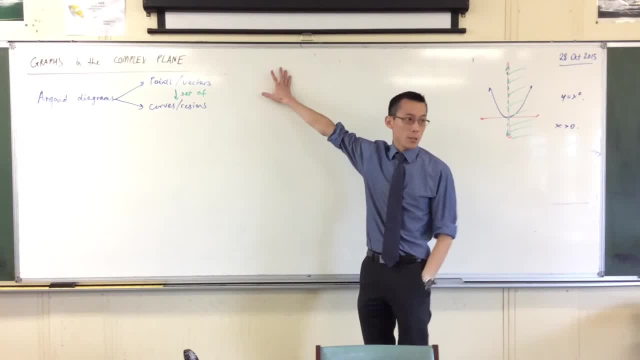 There is no reason why we can't do it in the complex plane. all right, But just remembering that when you think about points and vectors, we stop thinking about these, just as as, like numerically right, We start thinking about them. 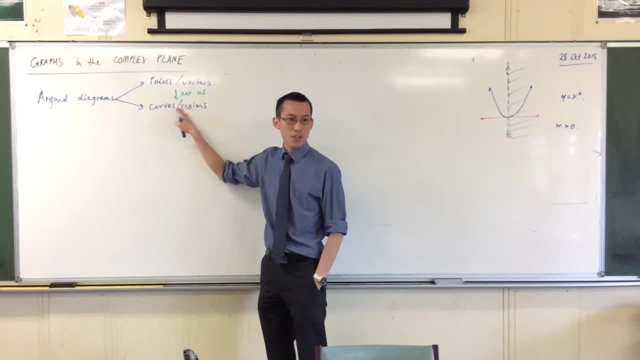 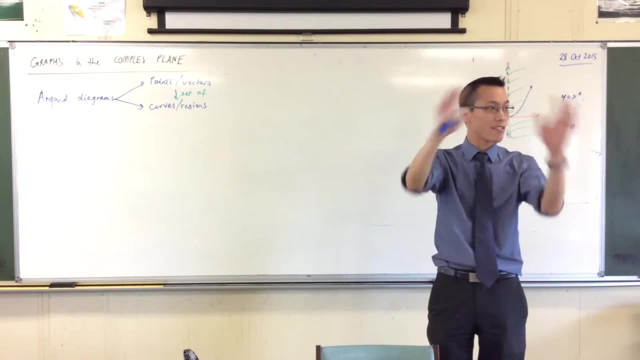 geometrically. So therefore, we're going to get things that represent geometry basically right Now. when we thought about geometry and graphing, we had a whole new set of ideas based around that and we called it locus right, So doing graphs in the complex plane. 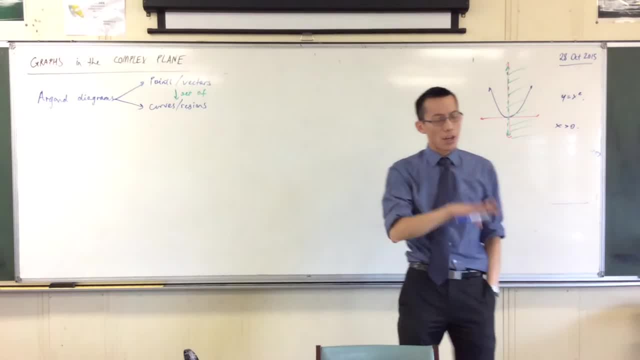 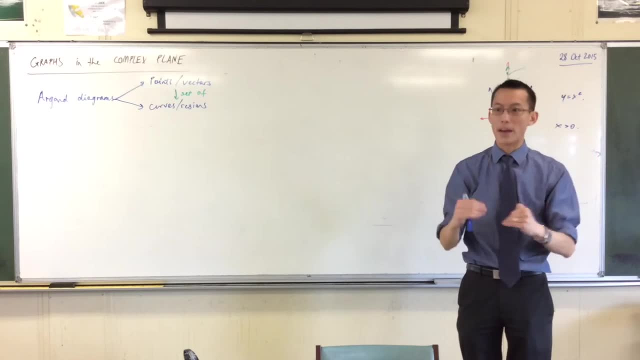 drawing curves and regions on an Argand diagram, or determining the locus of complex numbers that fit a certain geometric pattern or rule. those are just three different ways of saying the same thing, all the same idea, okay. So let's have a look at some really simple examples first, 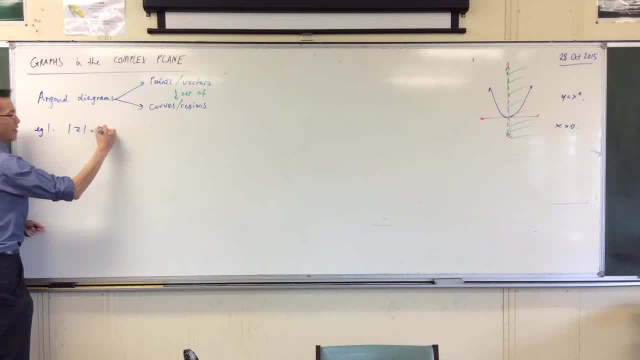 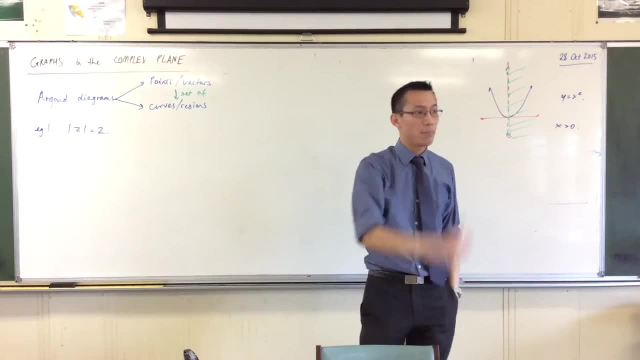 We'll begin right down the bottom of the ladder. Okay, so here, just like here, right? I'm not just giving you one complex number, I'm asking for all of the complex numbers that obey this property. okay, Does that make sense? 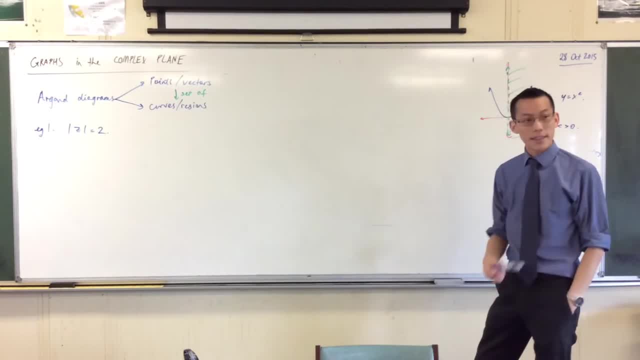 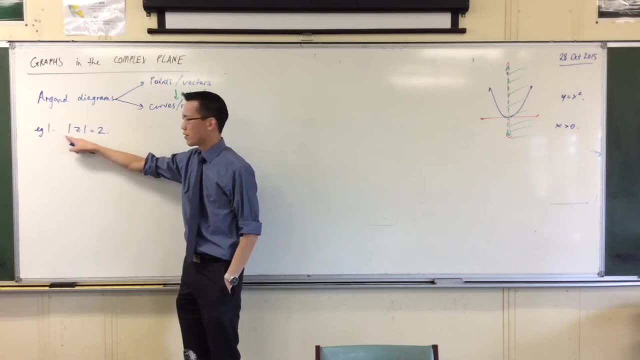 Okay now we can think about this in a variety of ways. We can think about this algebraically, we can think about it geometrically. I'm going to do both, okay? The absolute value, the modulus of z- What is that? 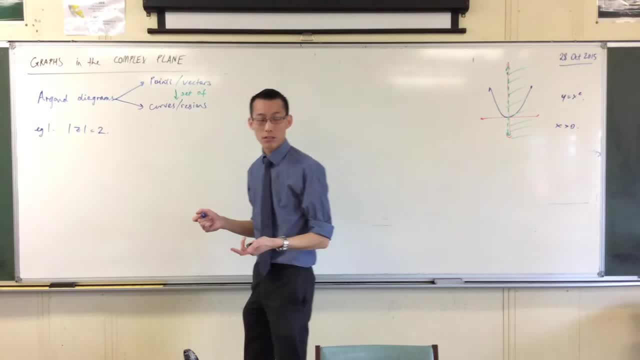 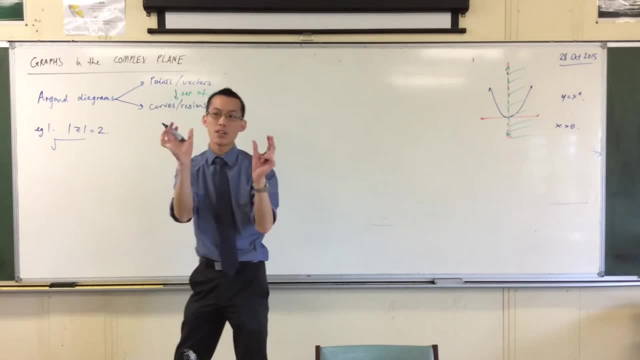 Like, if z is x plus i y, how do I calculate the modulus of z? I'll give you a clue. Starts with that: x squared plus y squared. I'm taking those coefficients of the real imaginary parts right. So I've got this. 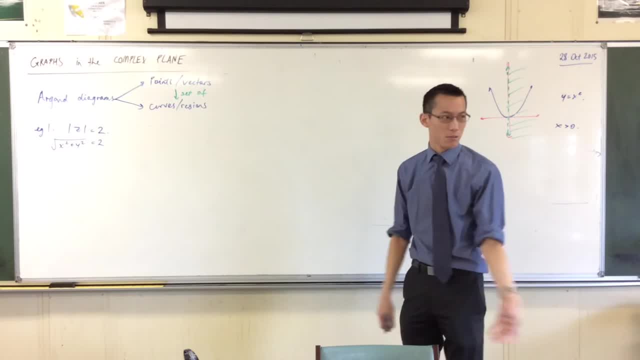 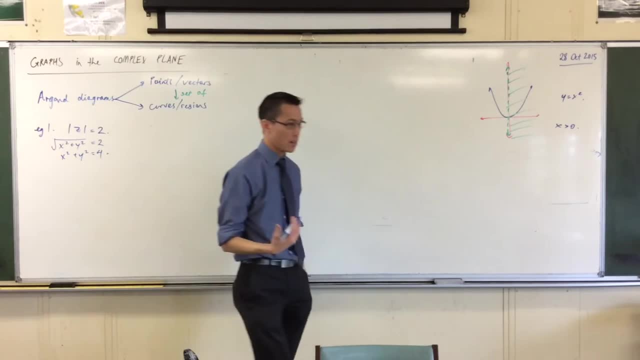 like: so okay Now, if I want to graph this thing, well, I guess I should probably square things out. so it's nice and simple, and I know exactly what this shape is. This is a circle with center at the origin radius. 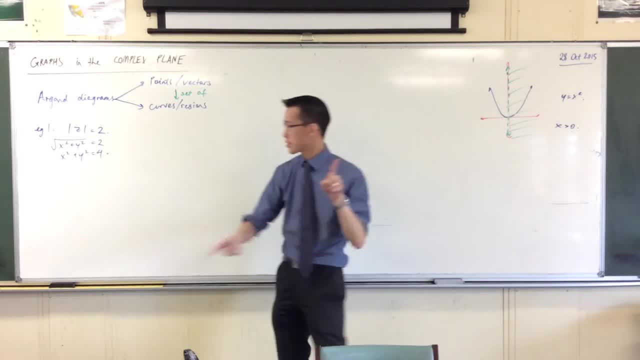 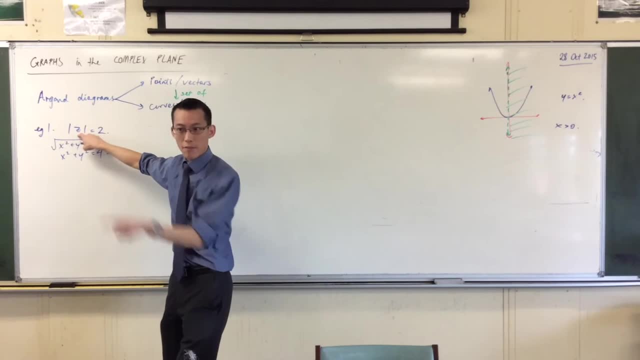 two, okay, Which of course we ought to have expected, because what does this mean geometrically? This means our distance from the origin. I want that whole set of points whose distance from the origin is two, which, of course, is this circle: okay. 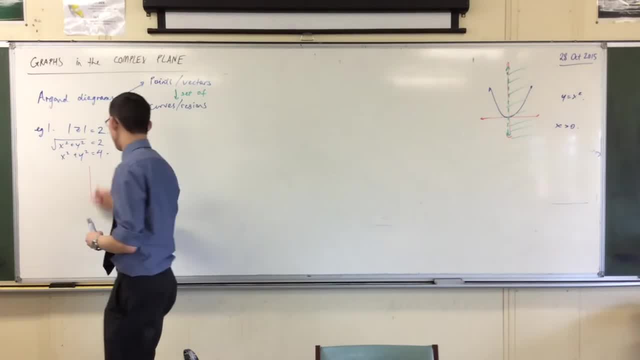 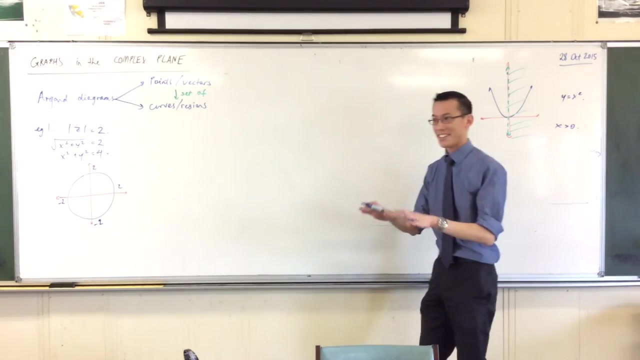 So let's just quickly draw it. okay, It's just a simple one to begin. So then we can just do the same circle. No, Okay, Well, isn't it? because absolute value is plus minus two? okay, You, okay, Yeah, All right, Now just think about it, right, What this means. 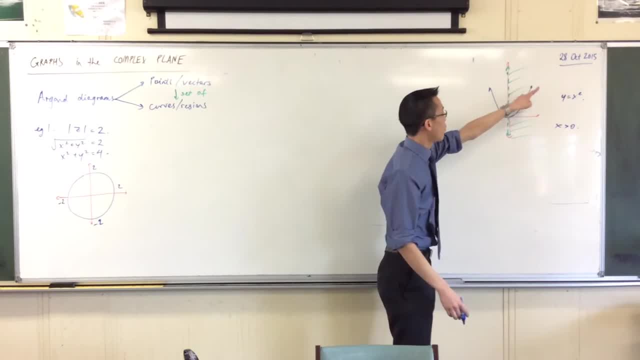 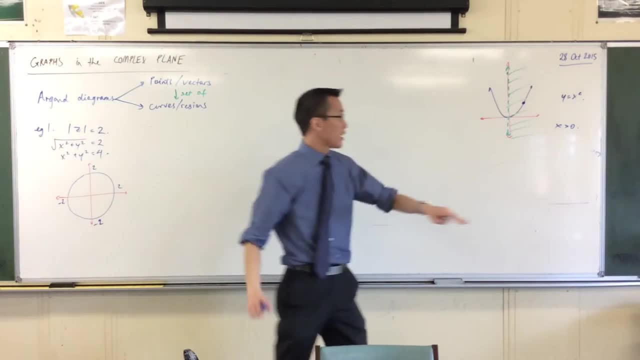 I'm gonna come back over here. What this means is that I can pick any point on, say, this blue parabola, right Point, like say: here I can take its y-value and I can take its x-value, and they will satisfy this equation, right? 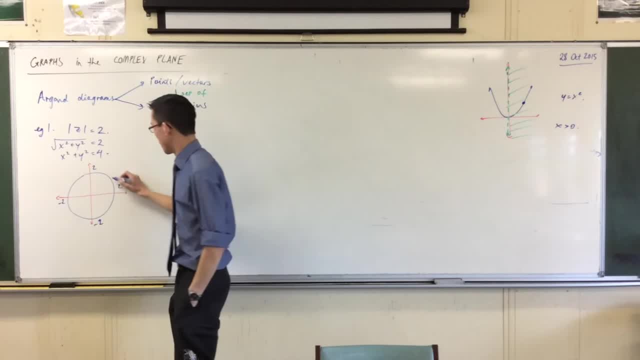 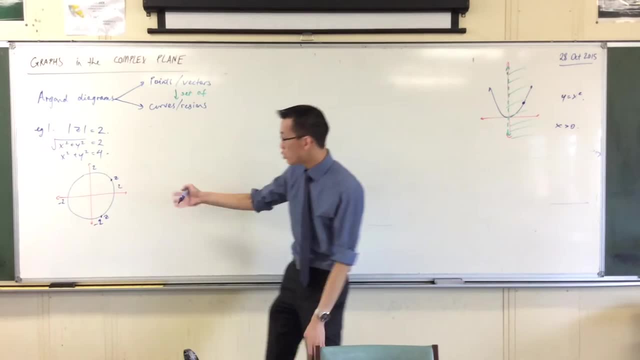 Over here. I should be able to take any of these coordinates, like: let's put z there or put it here or anywhere else you'd like, and if you take the modulus of z to that point, you'll get 2, right? Does that make sense? 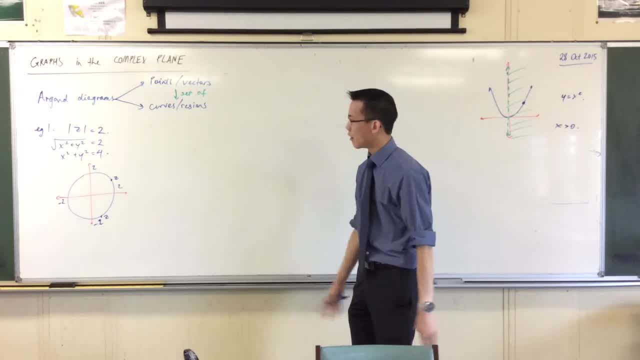 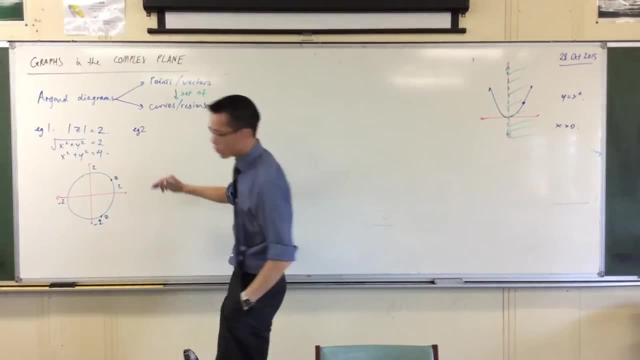 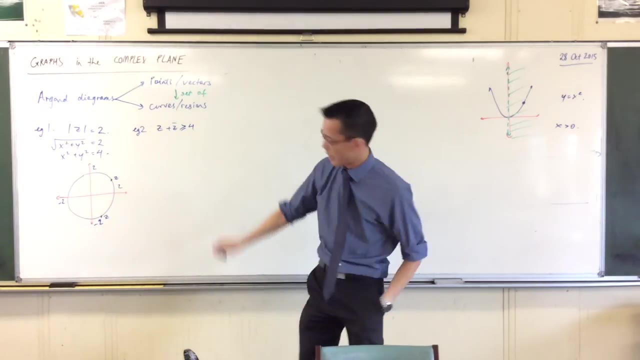 So that's all we mean. That's not complicated. That's like: oh, this is pretty, this is pretty calm. Let's have a look at another kind of example. Let's say: we'll do this one. Yeah, let's do this. Actually, I'll exclude the matter. 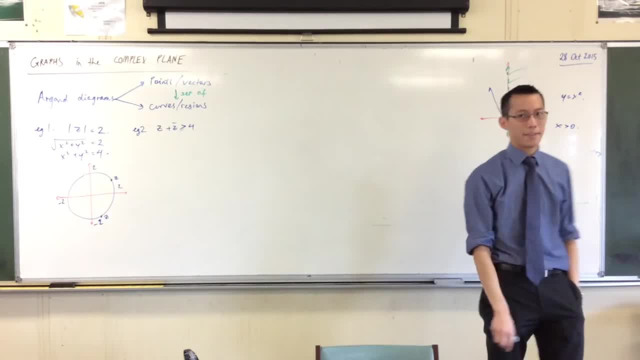 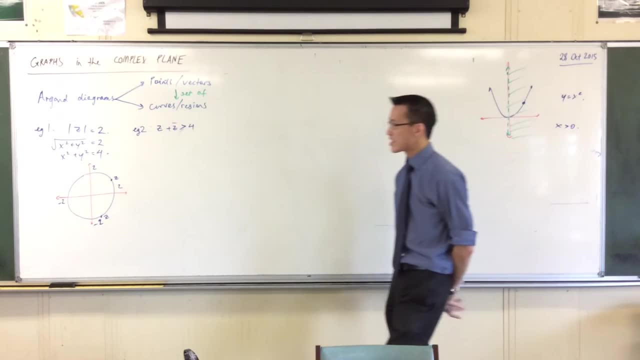 That's a little more interesting. Okay, what does this mean? Well, this is a little trickier to think about exclusively geometrically, but not that much harder. Let's think about the algebra first and then see what that tells us about the geometry. 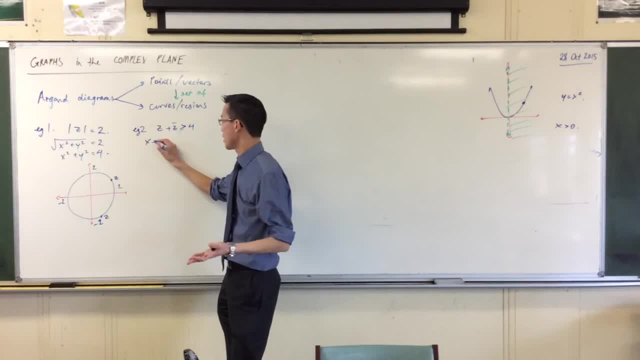 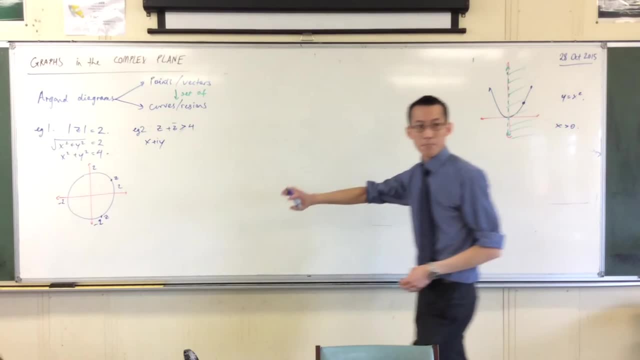 Z is a complex number. By definition. that means it's got a real and an imaginary part. Z bar is the conjugate, which means in this particular complex number it's going to be X minus X minus. good, Now we've noticed. the important thing about conjugates is that when you 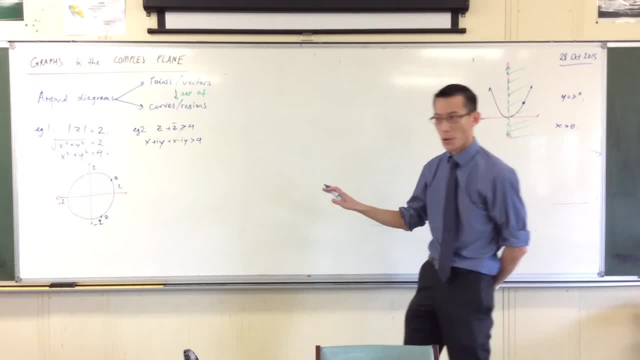 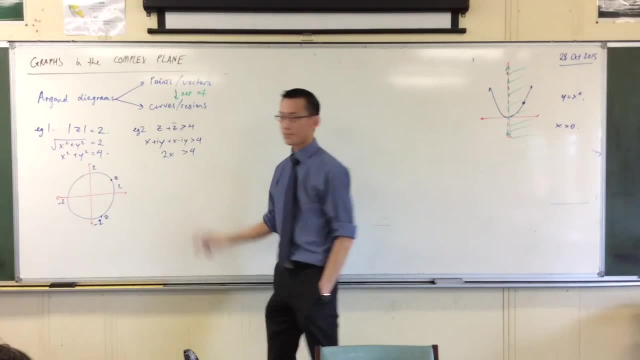 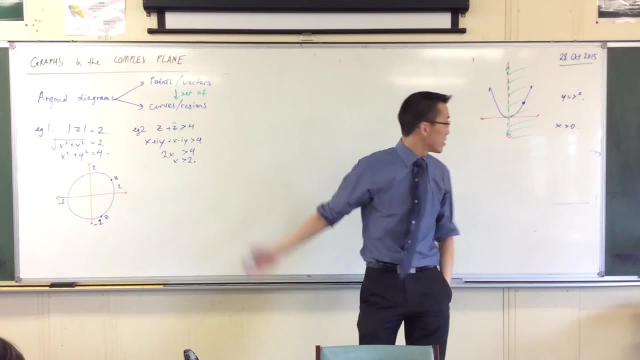 do lots of operations on them. all you get left with is the real component, right? So you can see my two imaginary parts here are going to cancel. That gives me this, And then all I need to do is divide through. So I know how to graph this. In fact, I almost did just over here. 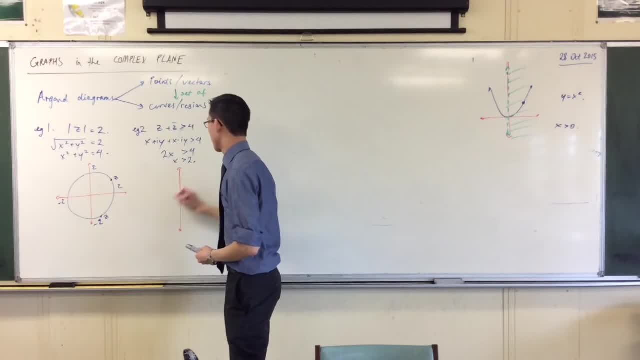 I just need to shift it a little bit. Let's draw it. It's not inclusive of the boundary, so I'm going to put a dotted line in. So I've got a boundary: x equals 2.. And then everything over here, every complex number over here. 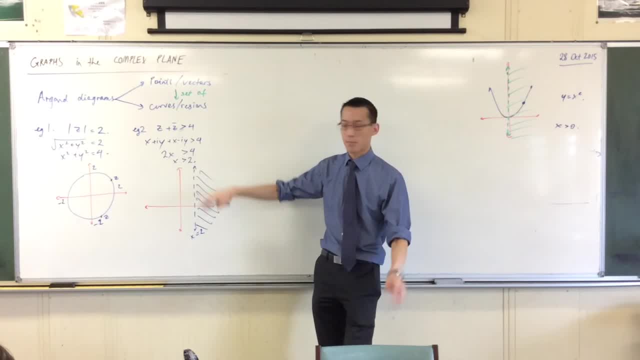 has a real component that's bigger than 2.. That's simple, right. By the way you can notice, I could have just as easily said, could just as easily have stated that as the real component of z being greater than 2.. 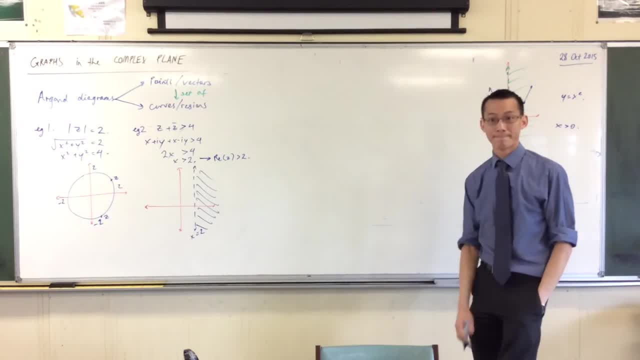 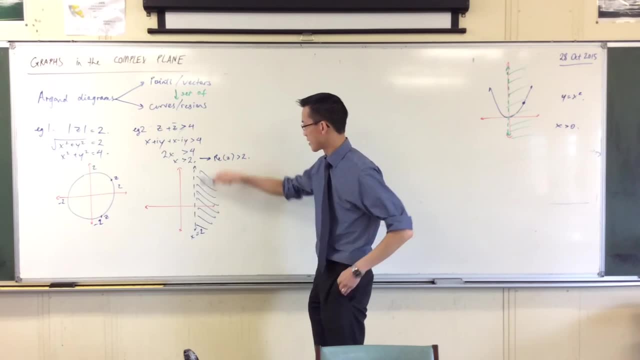 But do you see how those are the same thing. It's just different notation. It might not be related, but you see how the dotted line you drew. there's the arrow at the top and the bottom. Yeah, Is it essential to have those arrows, do you think? 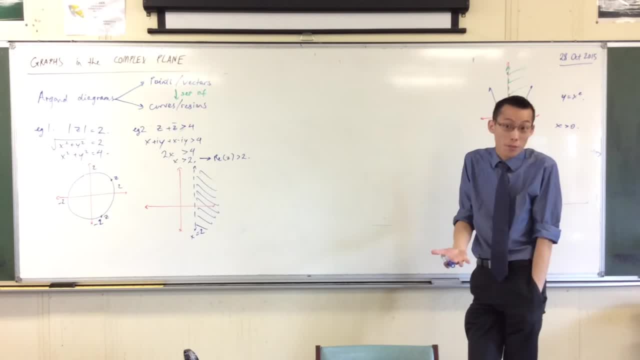 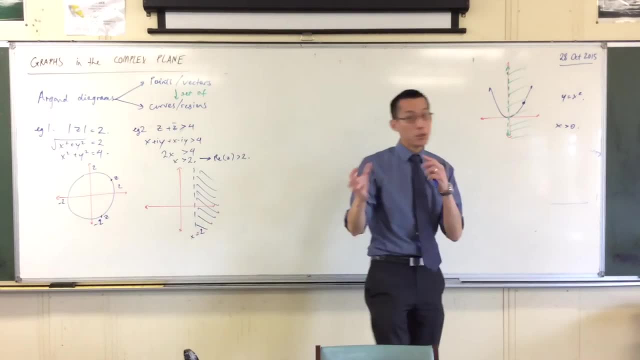 I wouldn't think of any reason why you wouldn't, because it does go on forever In some ways, if I had, not, being that there's no filled or hollow circles, that also kind of implies that it's going forever, because I've never said it stops. 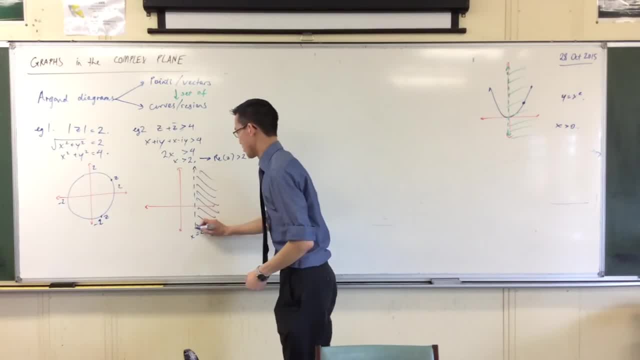 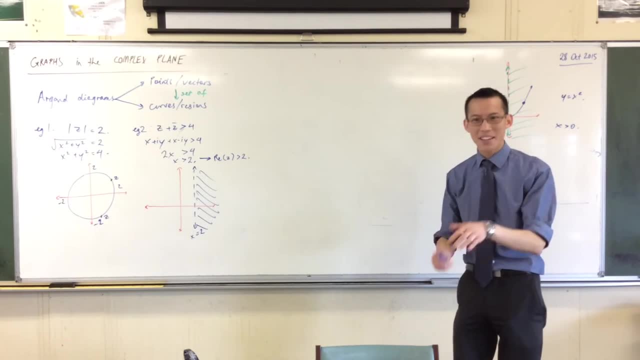 But being that I mean that it's going to go on forever, I don't see any reason not to put them there. Would it also imply an asymptote if you did Wait? no asymptotes, you draw them. OK, Asymptotes are a bit tricky. 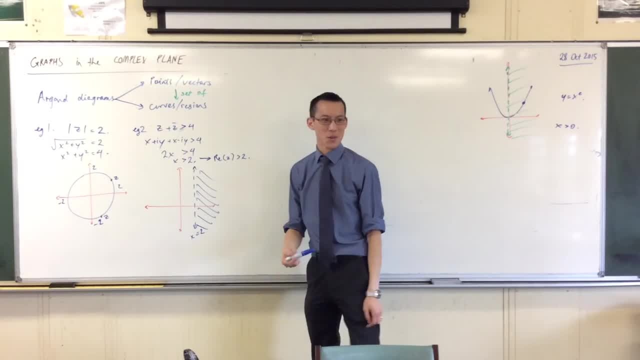 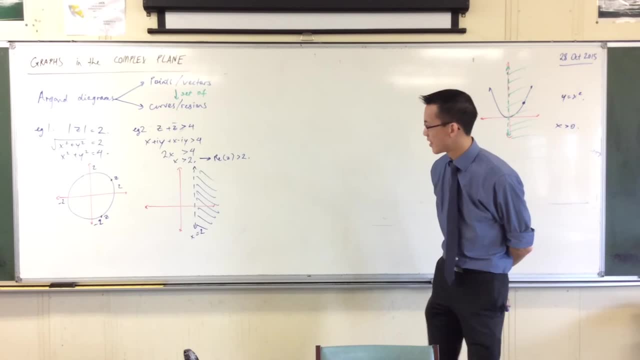 That's where we start to get out of. how many different ways can I draw a line to indicate it's a line, but it's not a line? that's on there. Yeah, I think that's fairly unambiguous. So over there you said x and reals are pretty much the same. 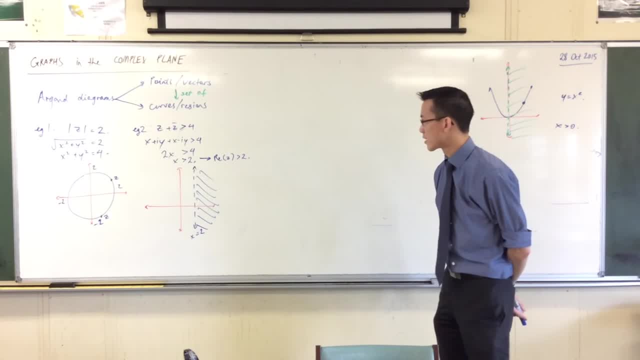 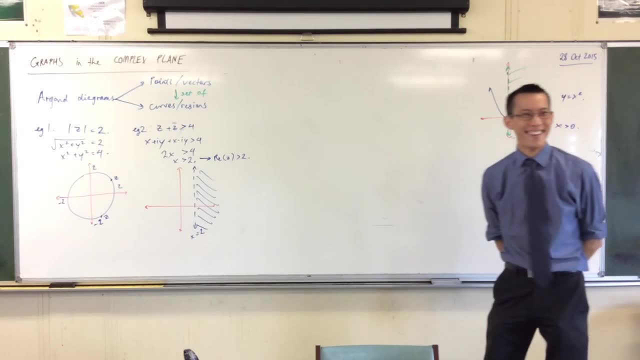 Yes, So when you label the axes, can you write x and y instead of imaginary and real, Because it's x plus i, y? That's a great question. I'm going to In a real. I was going to say in a real sense. that makes sense. that makes sense. 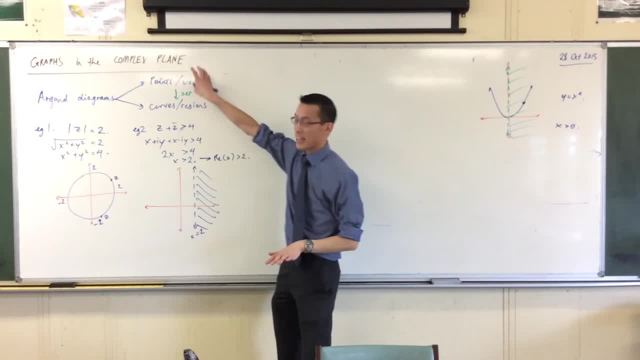 I'm not going to. I'm not going to because I'm strictly saying: this is the complex plane, Right, If I just say, if I just label this x and y, there's nothing there to indicate at the moment that there's any imaginary component to this. 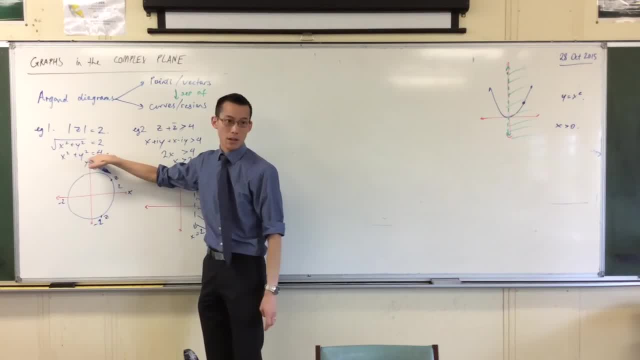 Right, For all I know, this is a real number and this is also a real number, Hence the Cartesian plane, not the complex plane, Right? So even though this is talking about y values, it's not just talking about y values. 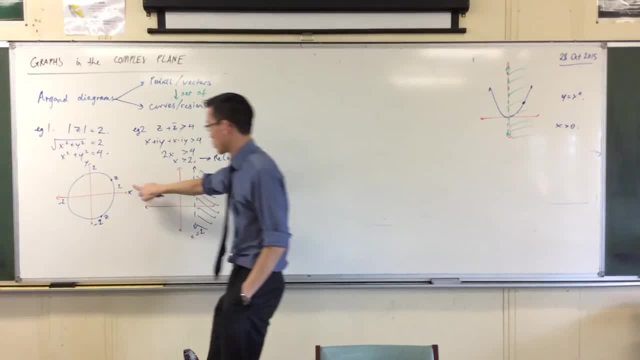 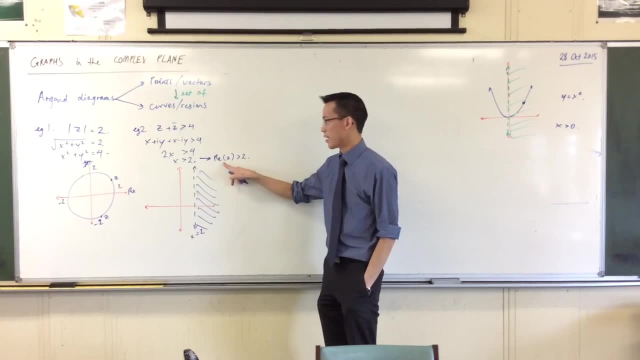 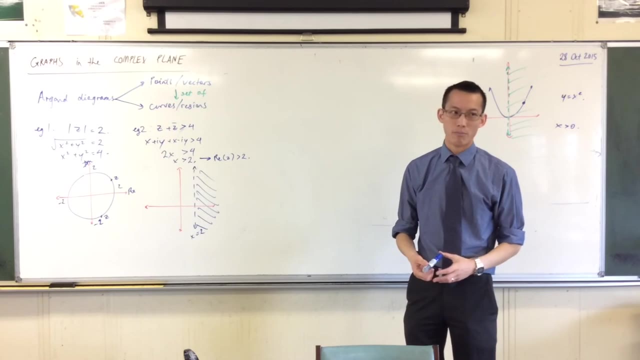 I'm specifying by way of the labels on the axes that these y values are not real, They are imaginary. Okay, So to say real z here indicates like the values, not the actual axis itself. Does that make sense? So I'm still going to call them real and imaginary. 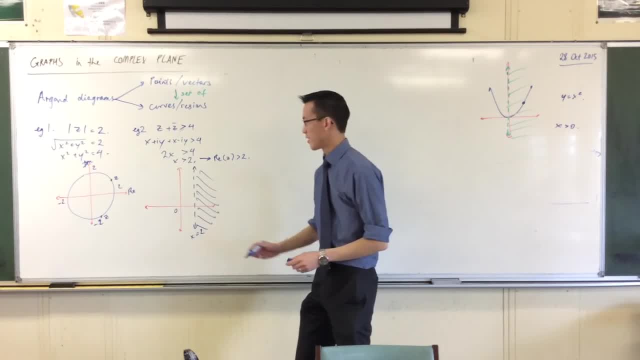 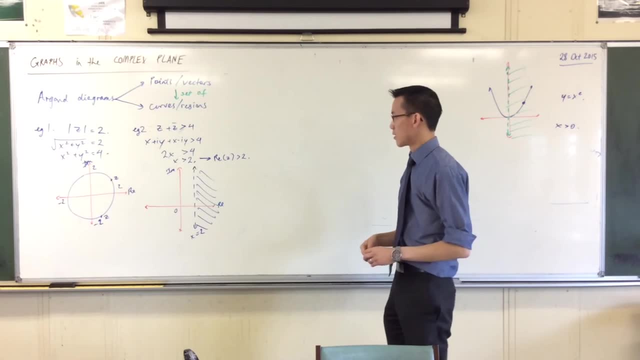 Okay, Yeah, Because whenever I draw this sort of graph right, and because there's no equation, there's no equal sign, I usually put a circle on the where x equals to 2.. Is that You mean here? Yeah? 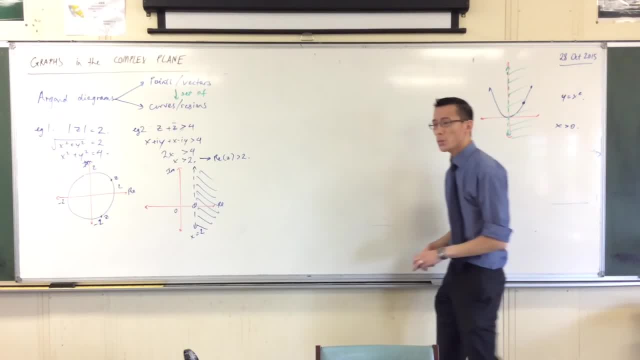 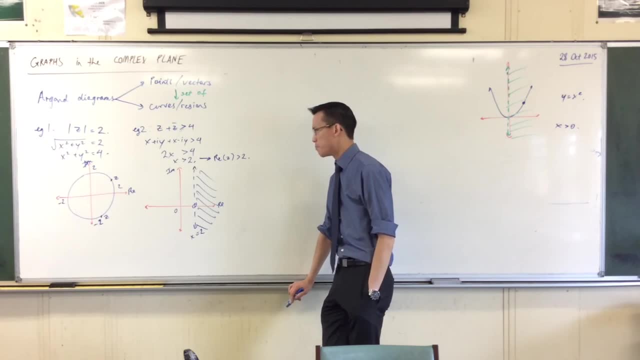 Like there, Yeah, An open circle there, Yeah, I mean, we'll get to where you need to include open circles and where you don't need to. I don't think there's anything. I don't think that takes away from the answer. 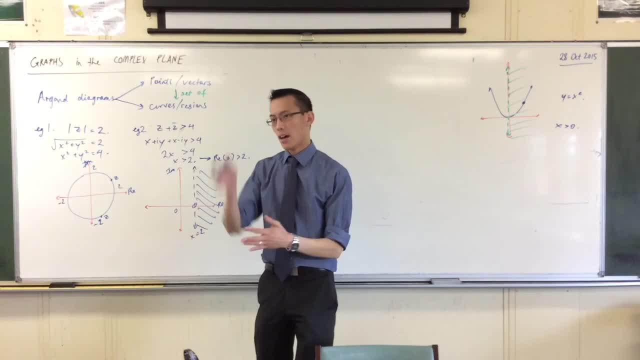 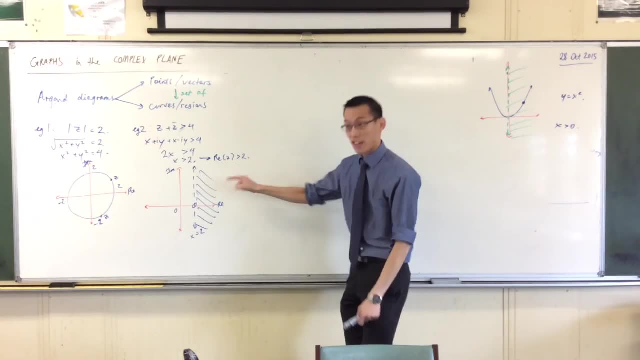 But I don't think it adds anything either. Like the dotted line already indicates, I'm excluding that boundary and I can't go on there. Okay, There will be points later on that we'll look at. Fingers crossed. You do actually have to specify that. 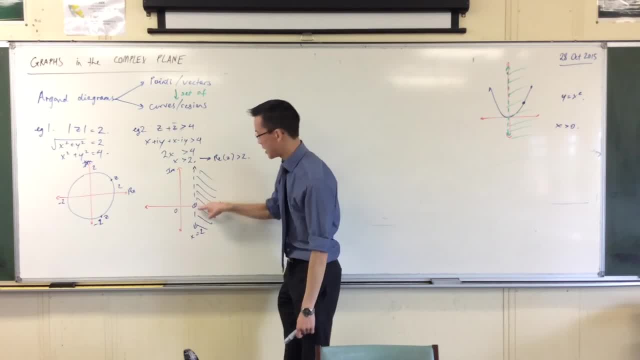 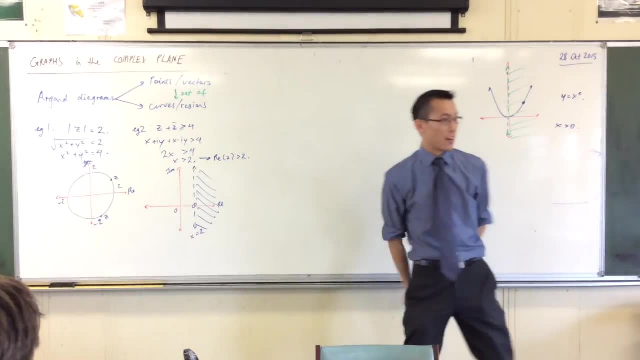 But you generally have to specify it where you've included the boundary, except for a particular spot, Whereas here my dotted line already excludes the boundary because it's a dotted line. Okay, Now, just really quickly, before we leave this diagram, let's just be a bit cheap. 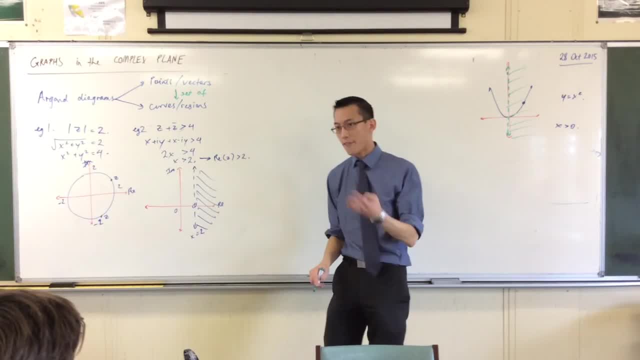 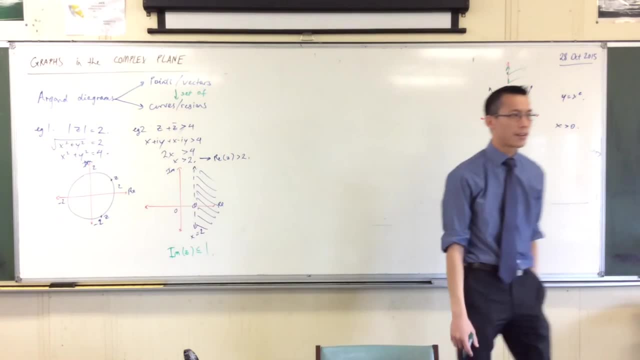 If I asked you, for instance, now that you know this, that these are equivalent, if I just said: okay, now graph for me this, where would that be? What would that look like? That's imaginary right. So that's my up down. 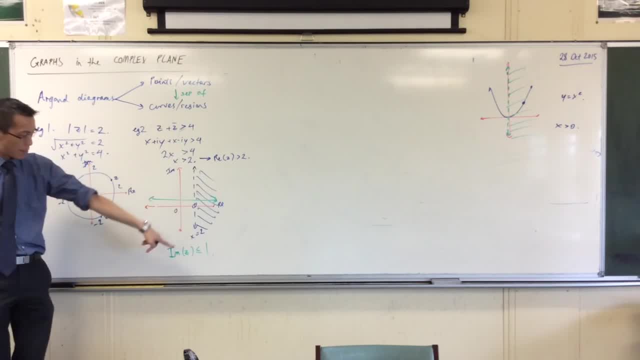 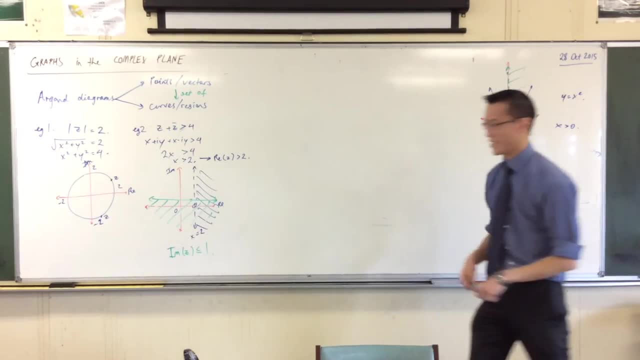 Okay, And you'd put in one, and then you'd say: notice, I've included my boundary. and then you say: everything I need, And so this is not a complicated idea. I almost said it wasn't a complex idea, But it is a complex idea. Just not that complicated Okay.